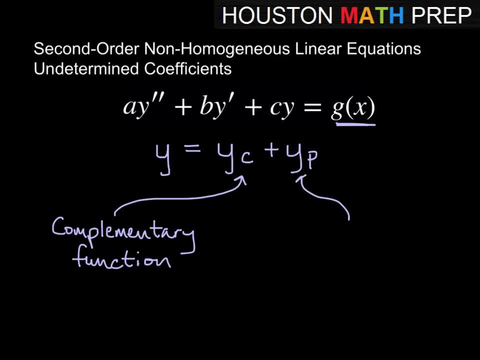 And then y sub p is going to be our particular solution That satisfies g sub x on the other side, and the form of y sub p is going to be based on the form of g of x. So let's say y sub p form is based on the form of g of x, whatever g of x is. 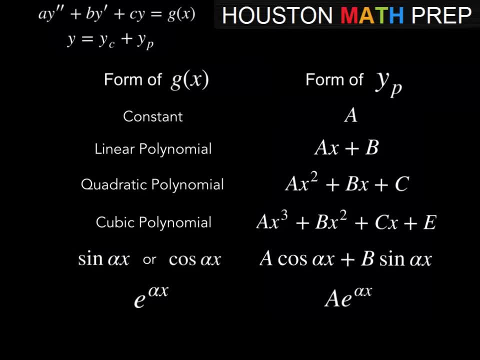 All right, I've written down most of the forms that we're going to find when we use this method. So if g of x is some type of polynomial including constants, or it's a sine or cosine function, or it's an exponential function. so you'll see all of the different types that we might get over here. 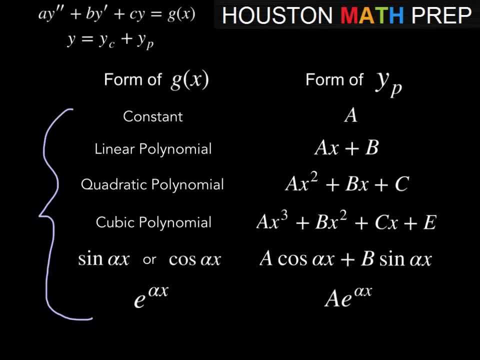 then the form of y sub p is going to be one of these listed here. So if our g of x- in other words, what's on the right-hand side of the equation- is going to be the form of y sub p, If our g of x on the right-hand side is a constant, then our y sub p is going to be of the form just a for some constant. 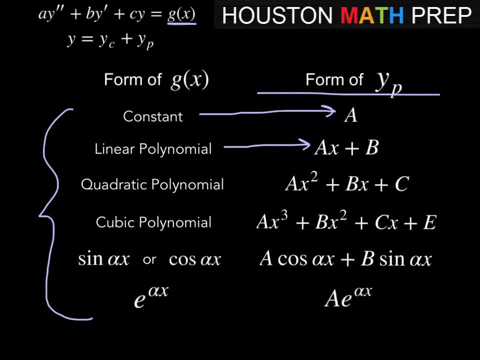 If g of x is linear, then y sub p needs to be linear, representing the first power of x plus the constant term Quadratic. if our g of x is quadratic, then y sub p must also be quadratic. Same with cubic, etc, etc. we could keep going with powers there. 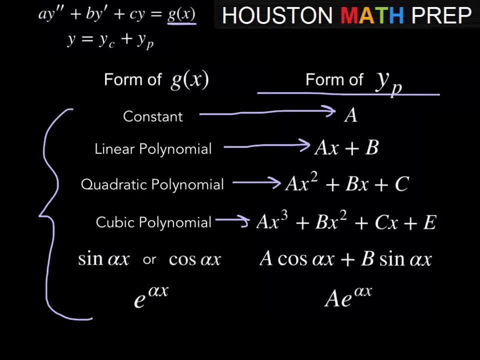 If it's some sine or cosine function, then our y sub p must also be quadratic. So y sub p will be multiples of the cosine and sine function. And if our g of x is some exponential, then y sub p will be some multiple of that exponential, with the same multiple of x there, same alpha. 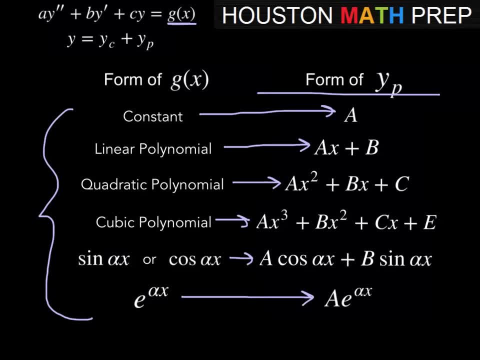 The idea is: when we have polynomials and we take derivatives, those give us obviously other polynomials. When we take sines and cosines, those give us obviously other sines and cosines. And when we take the derivative, 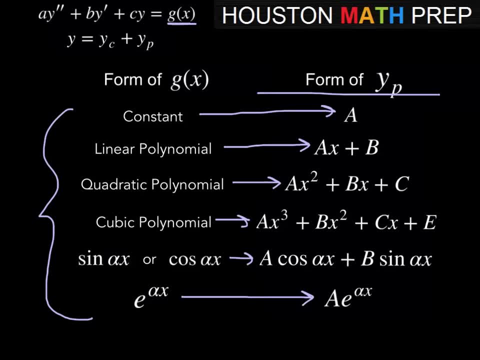 of exponentials, those also give us exponentials with the same expression in the exponentials. So these are all what you might think of as sort of closed under derivative in a way, in that when we take the derivative of one of these things we kind of get back something of the same form. 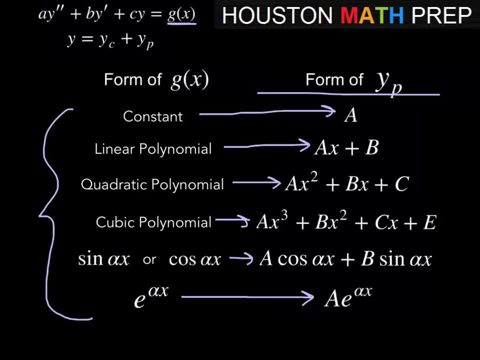 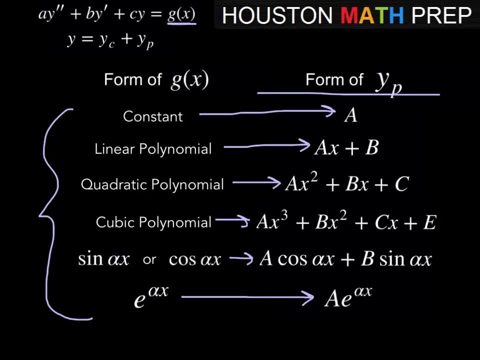 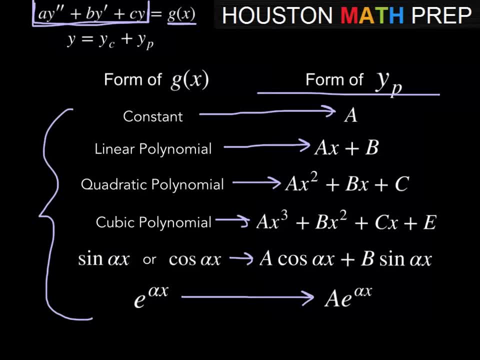 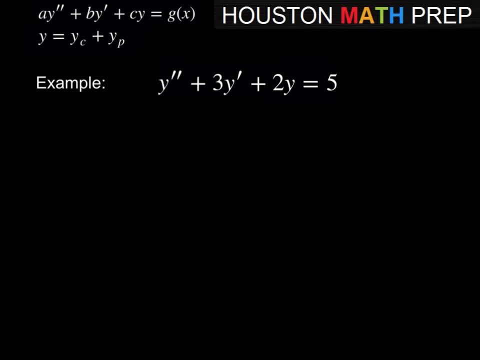 and then we'll go ahead and compare coefficients on the left and right-hand side and solve to get our y sub p, our particular solution there, And then we'll go ahead and compare coefficients on the left and right-hand side. Okay, so let's just start looking at some examples. 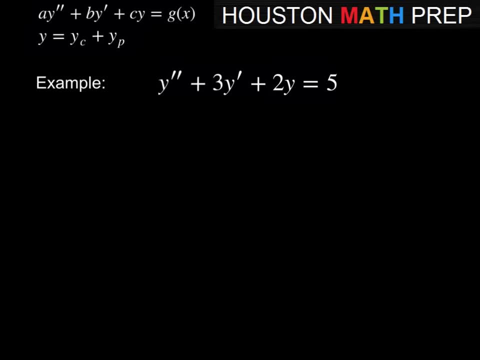 I'll start with the easiest one here. So what we would do is: first we would look at figuring out what y sub c is. first we would look at figuring out what y sub c is. first we would look at figuring out what y sub c is. 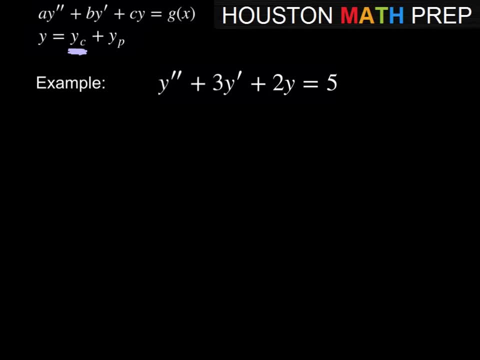 In other words the complementary function. That's done by using the auxiliary equation we get from the left-hand side, which would be m square plus 3m plus 2, equal to 0. So we'll set up what we would normally get from the homogeneous case. 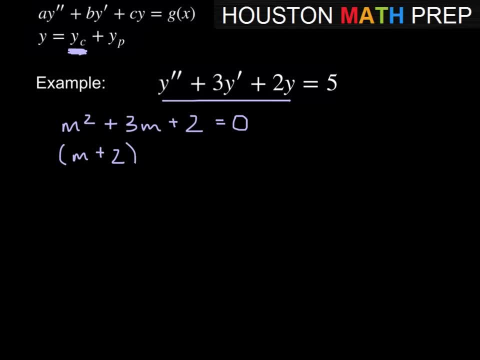 So that would give us m plus 2 times m plus 1 equals 0,. So that would give us m plus 2 times m plus 1 equals 0, which would then give us m is equal to negative 1 and negative 2.. 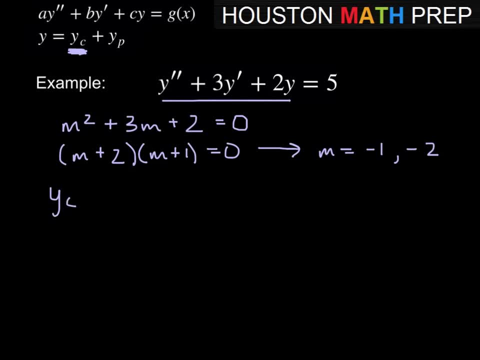 Those are the solutions. So we know that then y sub c is equal to c1 e to the negative x, plus c2 e to the negative 2x, based on those values for m here. Okay, so make sure you've checked out our homogeneous videos. 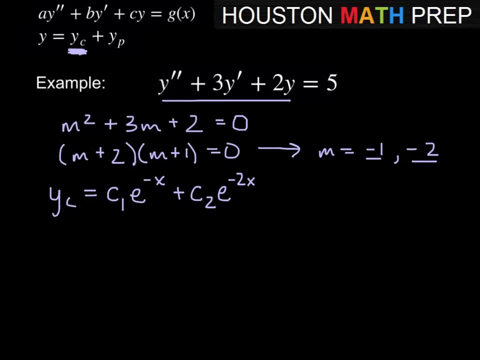 so you at least understand what we've done here with the auxiliary equation and finding y sub c. So the next part is finding y sub p. Okay, so y sub p is based on the form of whatever g of x is. Well, g of x happens to be 5 here, so we'll make a note of that. 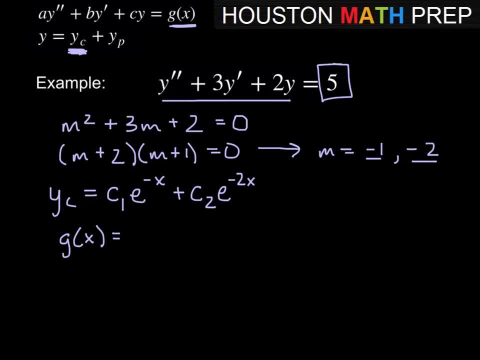 So g of x is equal to 5.. So if you need to rewind real quick, g of x is a constant. Looking back, then that means that y sub p is just going to be equal to a. to stand in for some constant. 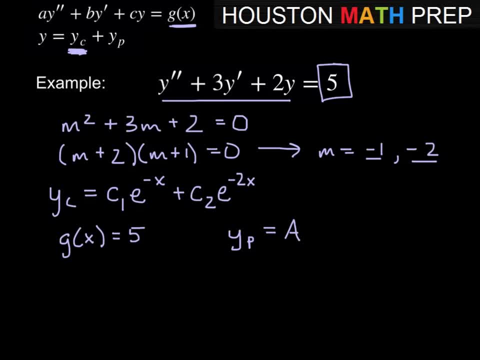 And what we want to do is we want to take the information we get and we need substitutions for everything on the left side here. So we have a substitution for y, We need a y prime substitution. We also need a y double prime substitution. 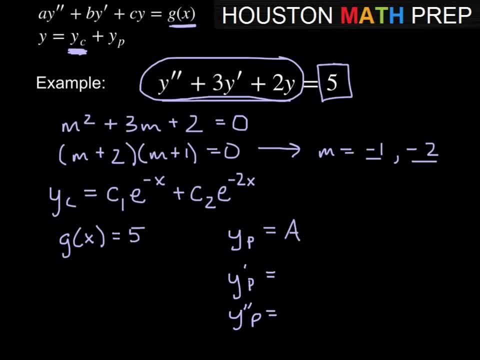 So if y sub p is a, which is a constant, the y prime of p would just be 0. The derivative of a constant is 0. And then the next derivative would also be 0. So we can take this information here. 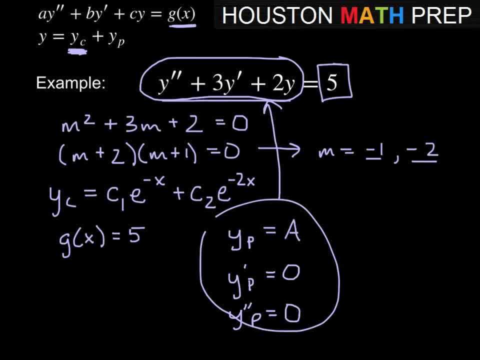 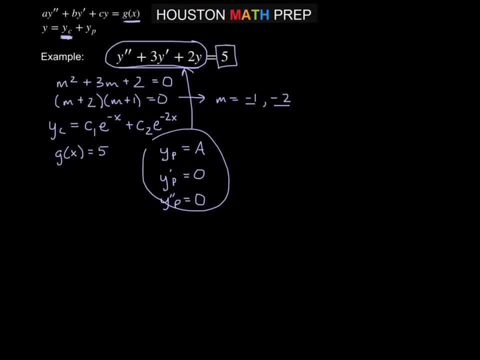 and we can plug it into our original statement equal to g of x and then begin to solve this. So let's go ahead and plug that information in. So y double prime is 0, plus 3y prime. y prime of p was also 0,. 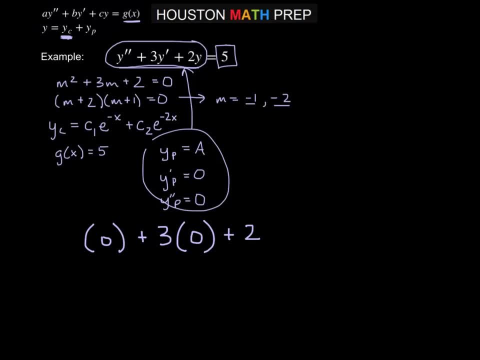 plus 2y, y sub p was a equal to 5, right? So I'm taking this information and putting it into the original equation now, and that's giving us this statement here. So we get nothing. nothing We get: 2a is equal to 5,. 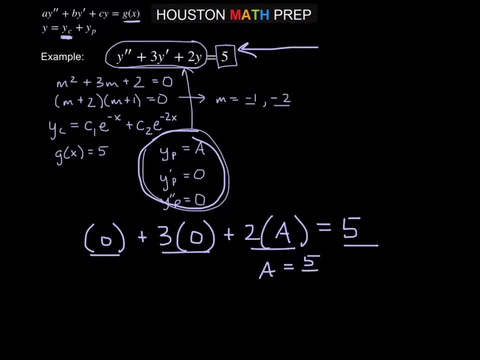 so that means a would be equal to 5 halves. Okay, And so our form for y sub p was y sub p equal to a. so we're actually finished here. So y sub p is equal to 5 halves, right. So now, if you'll notice, 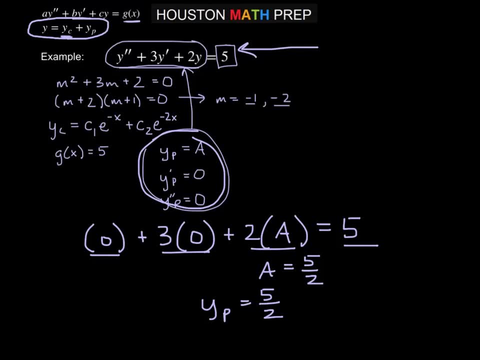 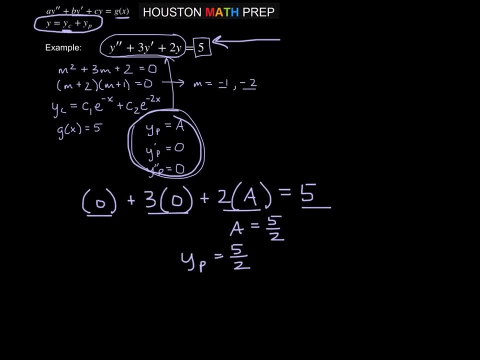 our solution will be: y is equal to the complementary function plus the particular solution. So our answer for this one is going to be: y is equal to c sub 1 e to the minus x, plus c sub 2 e to the minus 2x. 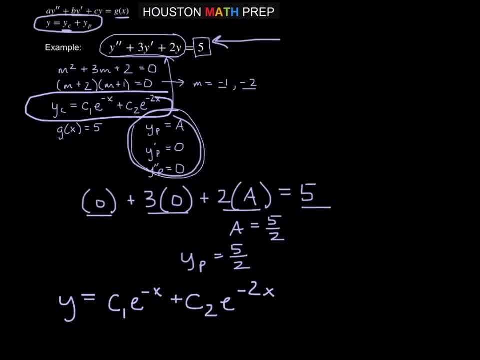 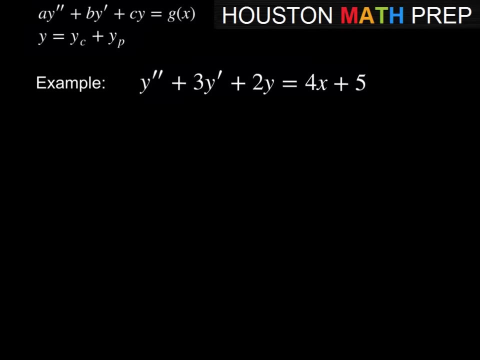 that was our complementary function plus y sub p, which we found was 5 halves. Okay, looking at another one here. so if you think about with this expression here what I'm doing is I'm keeping the same left-hand side of the equation. 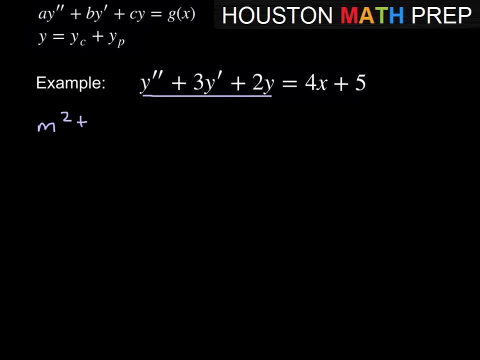 So we're still going to get the same m square plus 3m plus 2, equal to 0 when we try to solve for the complementary function here, y sub c. So we will get m equal to again negative 1 and negative 2.. 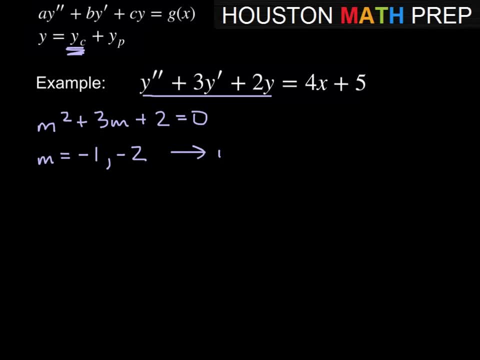 I'm not going to repeat the same work that we just did. So that would then tell us that y sub c is equal to again c sub 1, e to the minus x, plus c sub 2, e to the negative 2x. 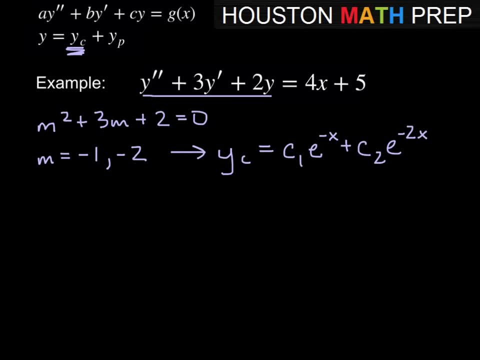 So I've sort of just I've left the left side the same, so that we don't have to do a bunch of extra work here, We can just focus on. okay, now the right side is different, So we need to figure out y sub p. 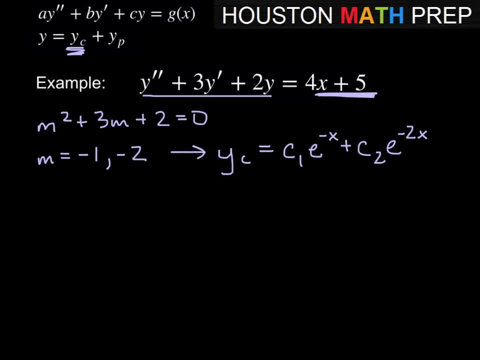 So we notice that g of x is 4x plus 5.. So now, instead of just a constant, we have basically a linear polynomial here. So if it's 4x plus 5, then that means y sub p is going to fit the form ax plus b. 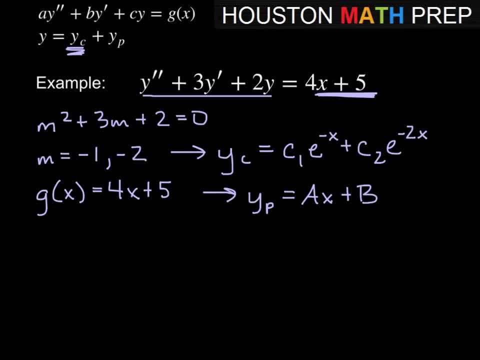 And now we're going to use this y sub p to find substitutions for everything on the left-hand side. So that's y. If we figure out y prime of p, then the derivative of ax plus b would just be a, And then the second derivative. 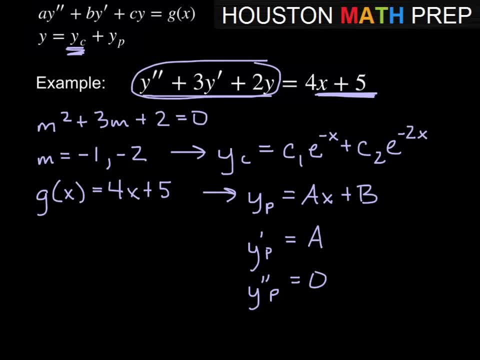 y sub p would just be 0.. Derivative of a would be 0.. So now we take all of this information, we put it in the left-hand side of the equation and then we solve. So if we plug in there, 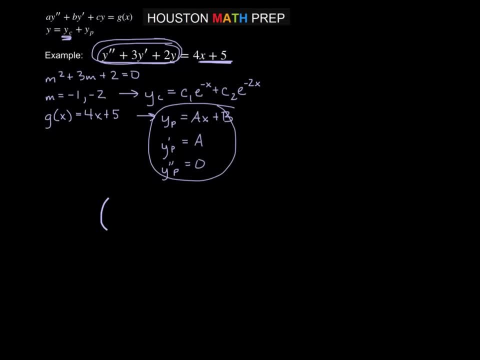 we get y double prime is 0 plus 3 times y prime, which is a plus 2 times y, which is ax plus b, equal to 4x plus 5.. Okay, so if we get nothing here, we get 3a plus. 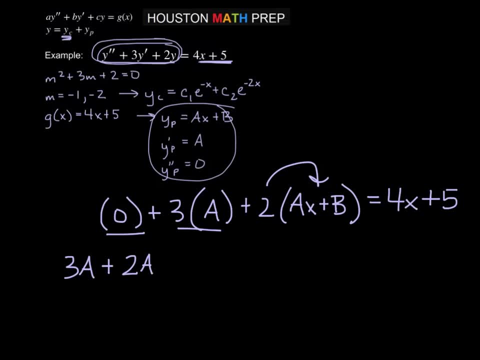 and then, when we distribute the 2,, we get 2ax plus 2b, and that is equal to 4x plus 5.. So now what I'm going to do is just group all of this stuff together, So we only have one x term. 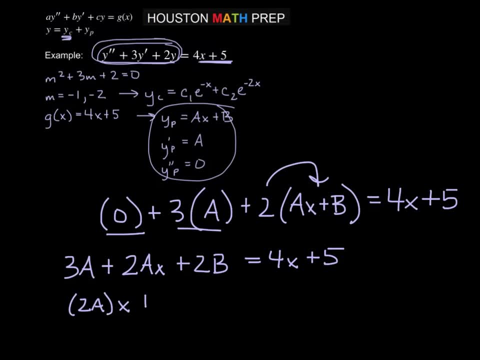 so we have 2ax, and then I'll group all the constants together: 3a plus 2b, and that's supposed to be equal to 4x plus 5.. And so now what we're going to do is compare the coefficients. 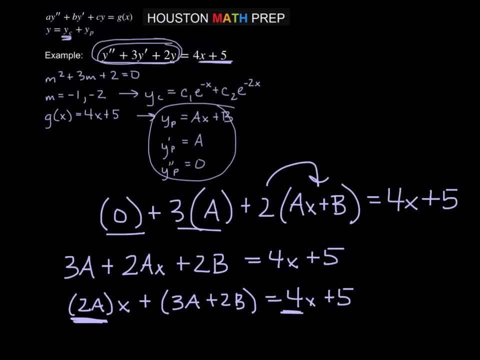 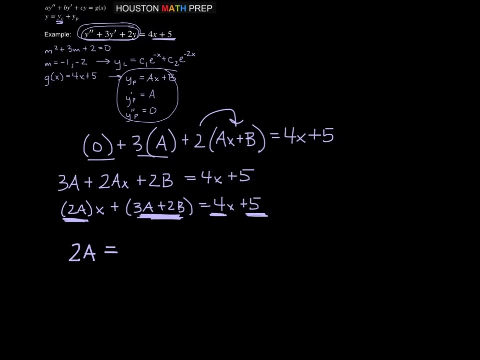 So we compare the x coefficient on the left to the x coefficient on the right, We compare the constant on the left to the constant on the right, helping us solve. So that then gives us the equation that 2a must be equal to 4,. 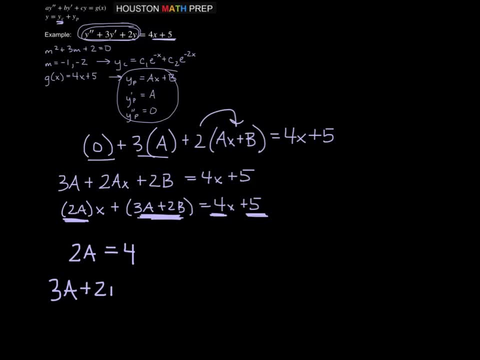 and 3a plus 2b must be equal to 5.. So the first equation is easy to solve. We divide by 2, we get that a is a is 2, and then we can take that information and plug it in down here. 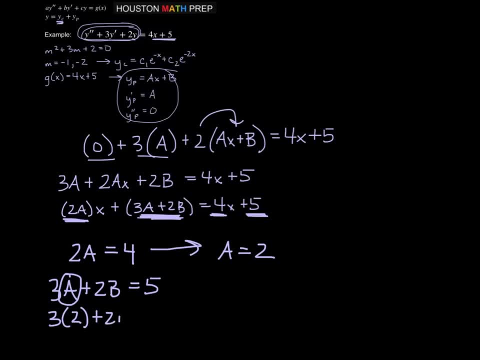 So we would get 3 times 2 plus 2b is equal to 5, and when we solve that we will get that b is equal to negative 1 half. And so remember, y sub p was equal to ax plus b up here. 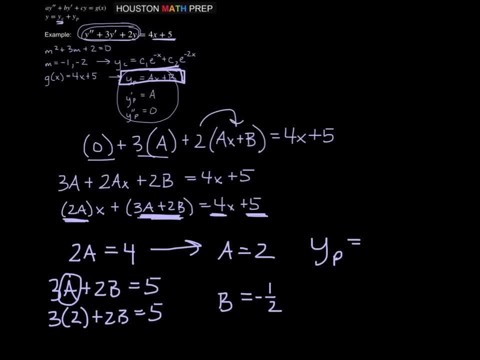 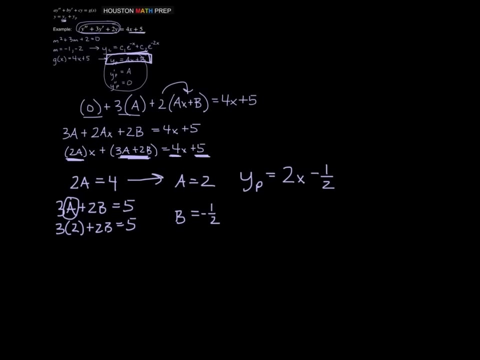 So that means y sub p. we now know a is 2, 2x plus b, so minus 1 half. So that's our particular solution. We combine that with our y sub c, which we already found. So y would equal c1 e to the minus x. 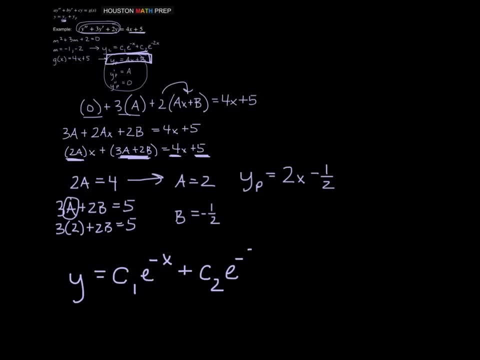 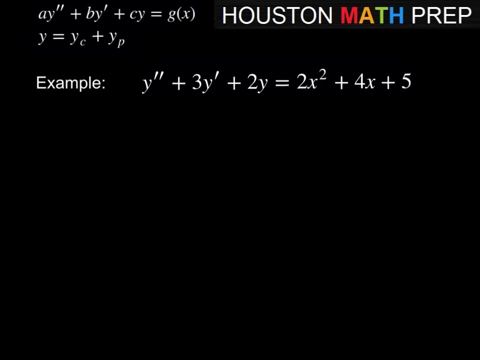 plus c2 e to the negative 2x, that's y sub c plus 2x minus 1 half, which is our y sub p. Let's look at another one that uses a quadratic polynomial. So again I've kept the left side of the equation. 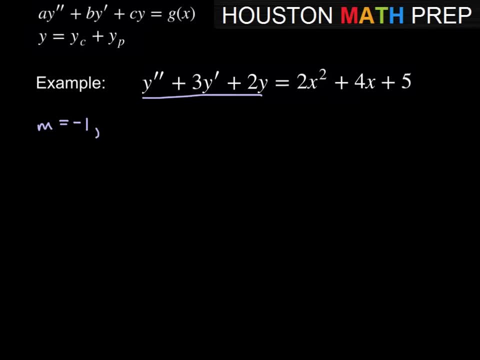 so we know from our auxiliary polynomial m is going to be negative 1 and negative 2, and that's going to give us that the complementary function would be c1, e to the minus x, plus c2, e to the minus 2x. 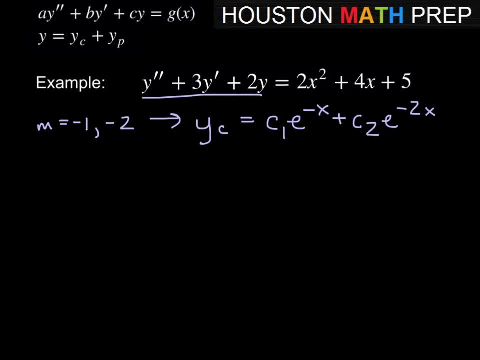 So I haven't changed anything about y sub c, because I'm using the same linear equation on the left-hand side. So now g of x is equal to 2x squared plus 4x plus 5.. So we need a y sub p with quadratic form. 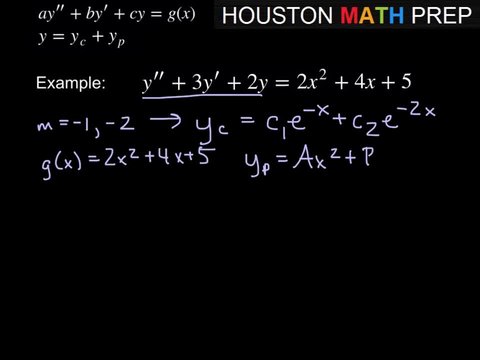 So ax squared plus bx plus c, And now we need information about the first derivative and the second derivative as well. So y prime of p is going to give us 2ax plus b, derivative of y sub p, And then y double prime sub p. 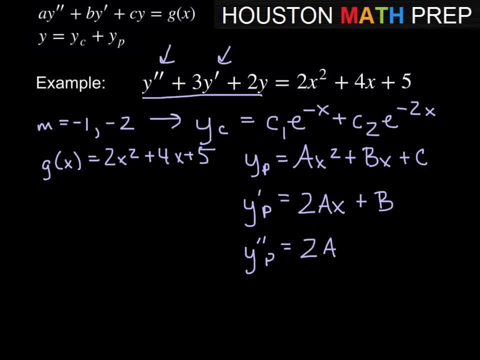 would give us just 2a there. So we're going to take this information, we're going to put it into the left side of the equation and then solve. So y double prime would be 2a plus 3y prime. 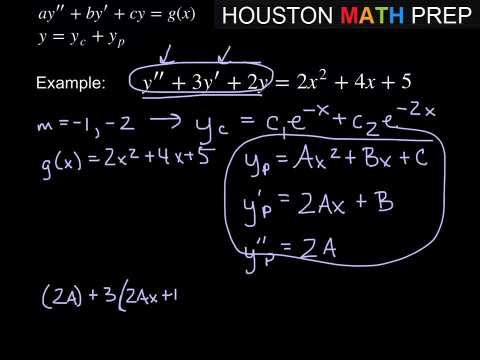 which is 2ax plus b plus 2y. so 2 times ax squared plus bx plus c is equal to: and then the right side of the equation, 2x squared plus 4x plus 5.. Okay, so now we need to then distribute. 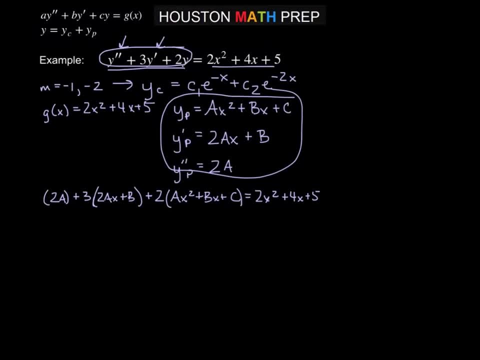 and compare both sides. So here we get 2a plus 6ax plus 3b plus 2ax squared plus 2bx plus 2c, distributing on the left hand side equal to 2x squared plus 4x plus 5.. 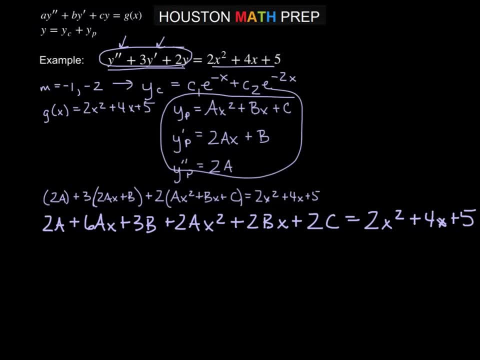 And then if we gather all of the terms, so this is the only quadratic term. so we have 2ax squared. that's how many x squared? we have x terms. we have the 6a here and we have the 2b here. 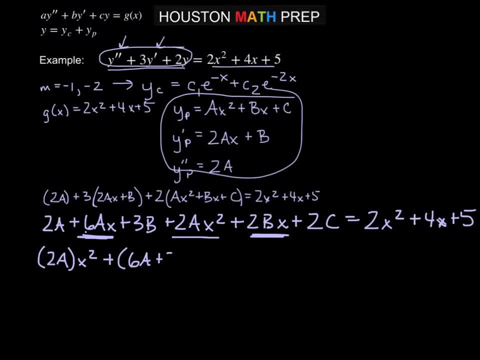 So we have 6a plus 2b- that's how many x's we have on the left side- And then 2a, 3b and 2c are all constants, so I'll group those together: 2a, 3b, 2c. 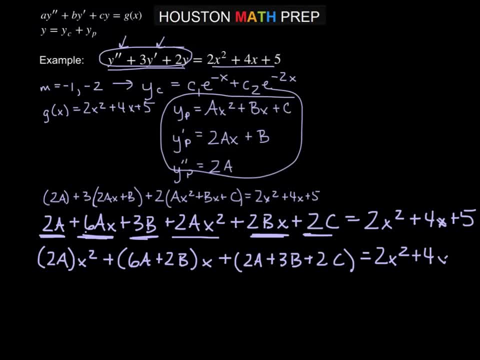 equal to our g of x. And now we compare the coefficients, So here 2a should be equal to 2.. And here 6a plus 2b should be equal to 4.. And the last one: 2a plus 3b plus 2c. 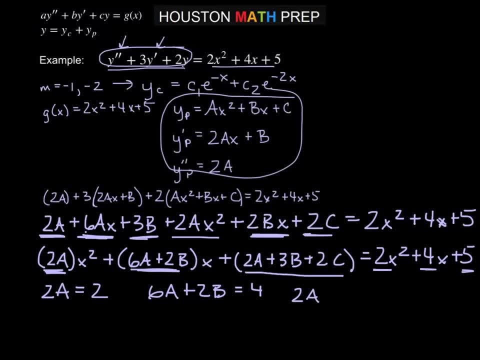 should be equal to 5.. Okay, so you start with the easiest one first. So solving this one over here, we should get that a is equal to 1. When we plug that in over here, we'll get 6 plus 2b is 4.. 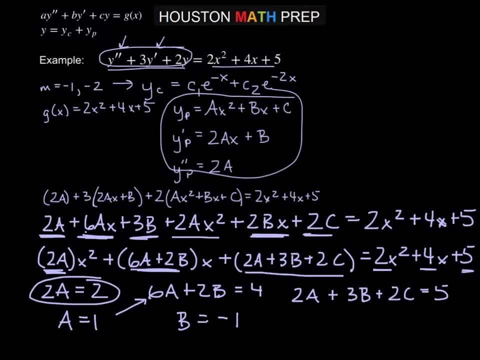 That would make b equal to negative 1 when you solve that, So plugging a and b over into this one would give us 2 minus 3, which would be negative. 1 plus 2c equals 5, and then you would get that c is equal to 3 here. 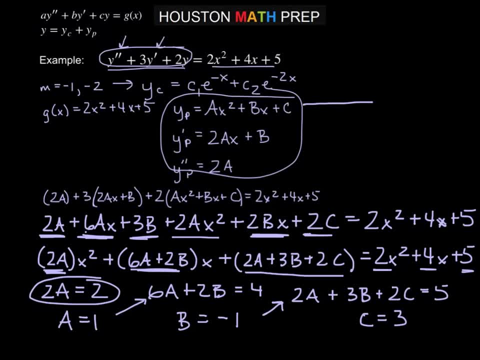 Okay, so you'll notice all that information can go into our y sub p, And so, in other words, y sub p is then equal to 1x squared b is negative, 1, so minus x, and then plus c, which is 3, so plus 3.. 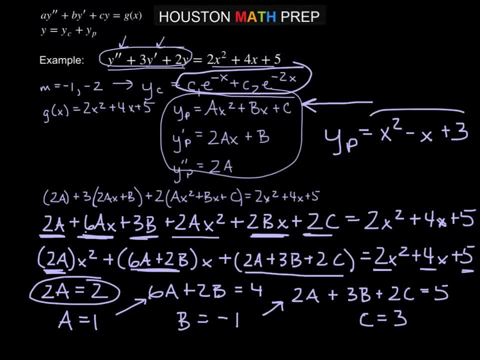 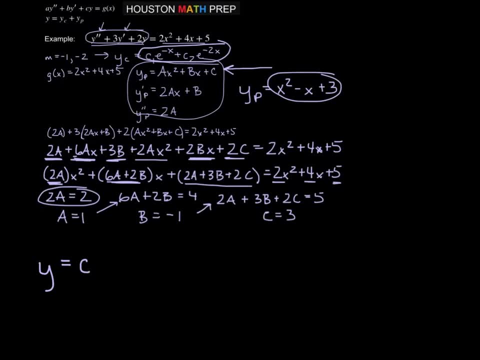 Okay, so we then combine our y sub c, our y sub p, and so for this one, that will give us that y is equal to c sub 1 e to the minus x plus c sub 2 e to the minus 2x. 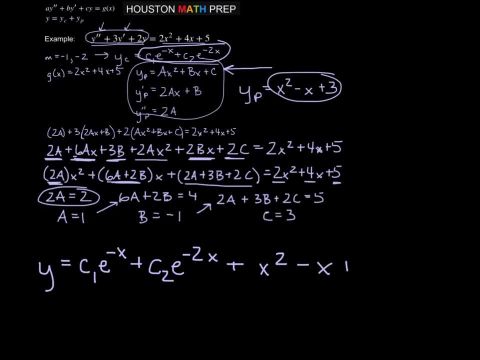 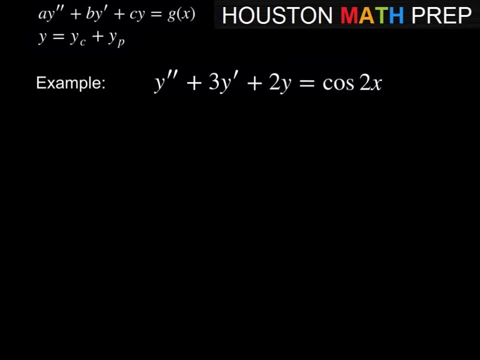 plus x, squared minus x plus 3.. Okay, let's look at a cosine example. So again, we're not always going to have y, double prime plus 3y, prime plus 2y on the left-hand side. I'm just using the same one each time. 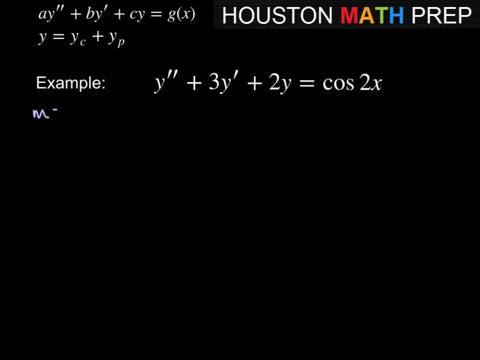 to make it easy for us to do So we know we're going to get: m is equal to negative 1 and negative 2 from that one. and we know obviously we've already said our y sub c- for this is going to be c sub 1, e to the minus x. 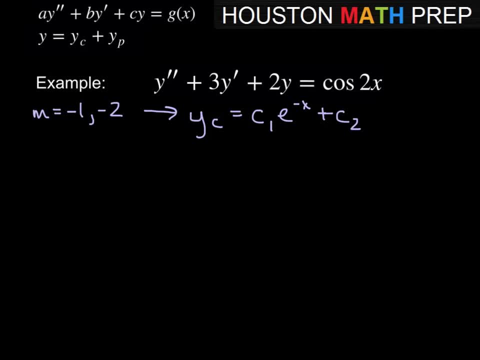 plus c sub 2 e to the minus 2x, So we've got our y sub c. That part's done. g of x is cosine of 2x, And so that then tells us that y sub p is going to be of the form. 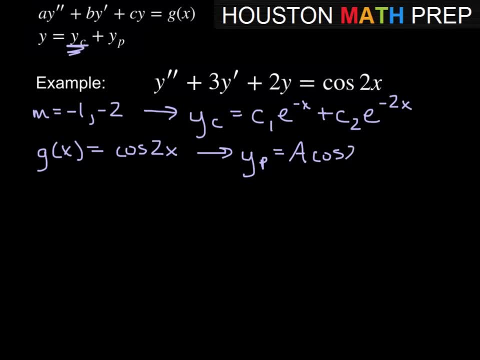 if we look back at the chart, a times cosine of 2x plus b times sine of 2x, That'll be our form of y sub p. That gives us a substitution for y. We need substitutions for y, prime, y, double prime. 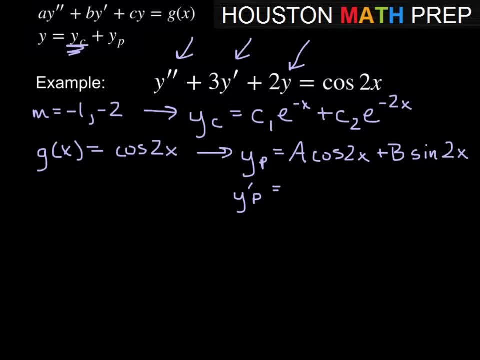 So y prime of p is going to equal negative 2a sine of 2x when we take the derivative of the first term plus 2b cosine 2x if we take the derivative of that second term there, And then we need the second derivative. 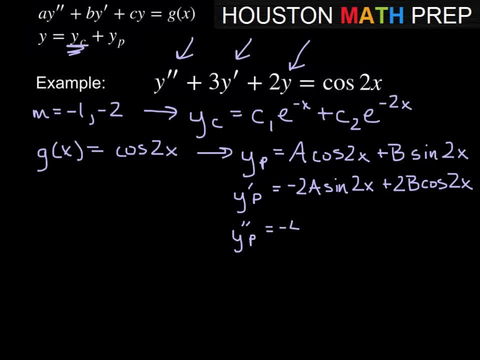 So y double prime p is going to equal negative 4a cosine of 2x minus 4b sine of 2x. Okay, so now we will take this information and plug it in here and see what we get for the equation. 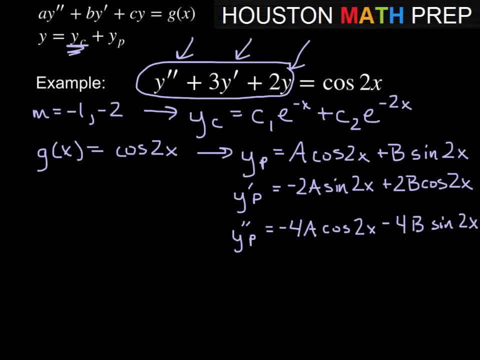 So this is going to take a bit of room. So y double prime, so that's going to be negative 4a cosine 2x, minus 4b sine 2x- Alright, plus 3y prime, so plus 3 times. 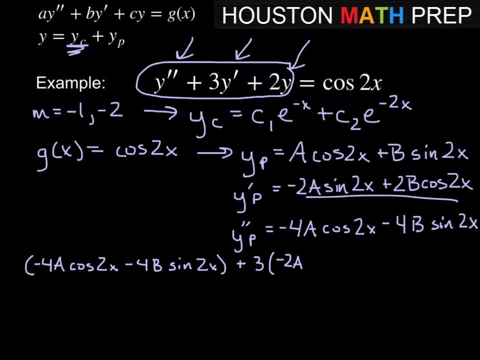 and then we'll put in our y prime information: negative 2a sine 2x plus 2b, cosine 2x plus 2y, so plus 2 times, and then we'll put in our y information: a cosine of 2x. 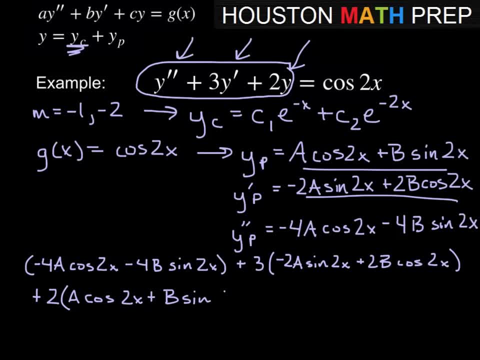 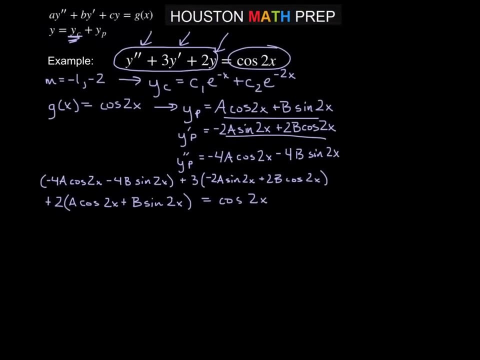 plus b sine of 2x, And all of that is supposed to equal cosine 2x. So I'm going to skip a little bit of the tediousness here and sort of distribute and gather all our terms in one shot. So once we gather all of these together, 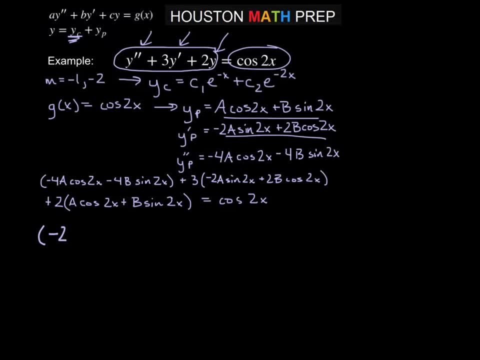 it turns out, I think we get negative 2a plus 6b, cosine 2x, once we gather all the cosine terms together plus, and then we would end up with, let's see, negative 6a minus 2b. 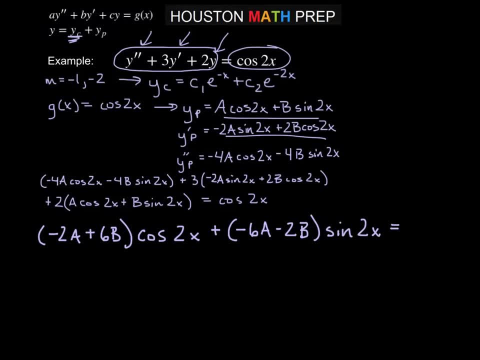 sine of 2x is equal to cosine of 2x, once we gather all the like terms And then we just want to compare. So you think about how many cosines we have on the left side. Well, we have negative 2a plus 6b of them. 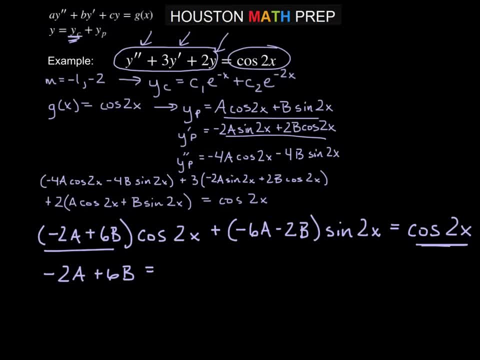 How many cosine 2x's do we have on the right side? Well, we just have 1, so that must be 1.. And then, when you look on the left side, negative 6a minus 2b, that's how many sine 2x's we have. 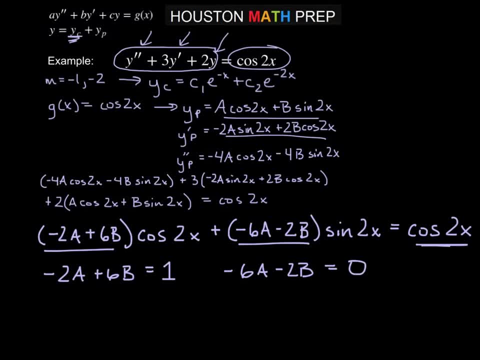 On the right side we don't have any sine 2x's, so that's actually going to be equal to 0 then, So this one's easier to solve, I think, and get a substitution. We have to solve both of these equations now. 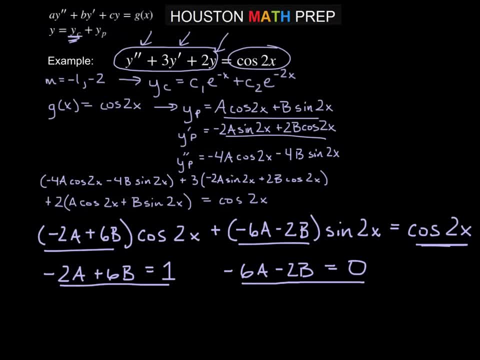 So we'll go ahead and solve. maybe I'll solve for b. So for this one here b ends up being- it looks like negative- 3a once we solve this one doing the arithmetic there And then if we plug that information in over there, 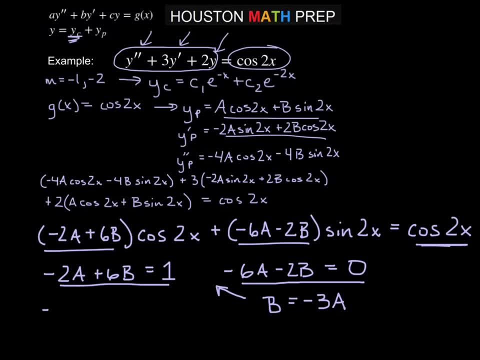 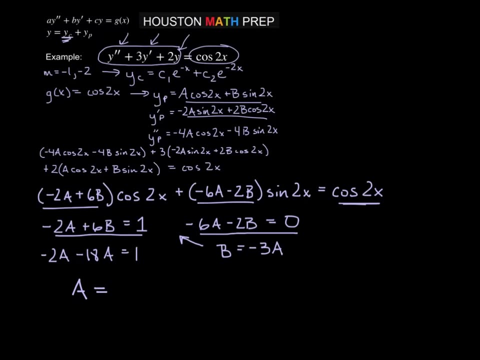 then we would get that negative 2a minus 18 more a's would equal 1. And I think that gives us then, when we solve that, a would be equal to negative 1 over 20. So we have something for a. 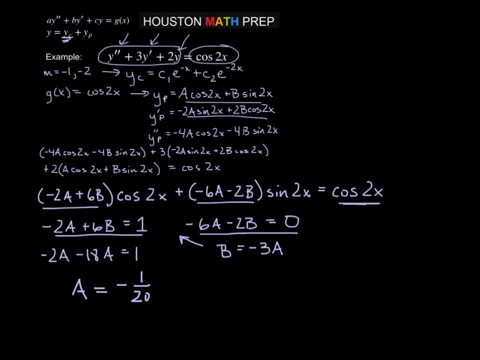 we just need to then find b. So if we take this information and plug it back in over here, we get that b is equal to 3 over 20.. Alright, and so now remember, our y sub p was of the form: 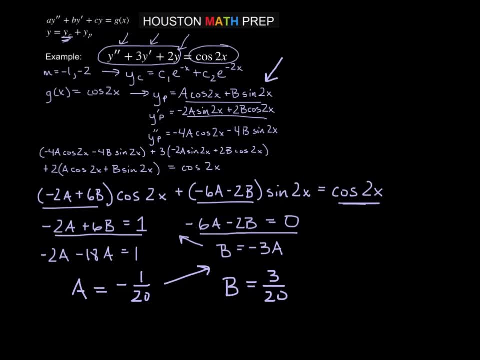 a cosine 2x plus b sine 2x. So that tells us: y sub p is equal to negative 1 over 20 cosine 2x plus 3 over 20 sine of 2x. And now, if we just simply copy that down, 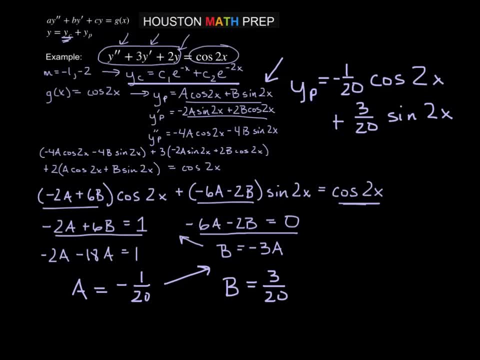 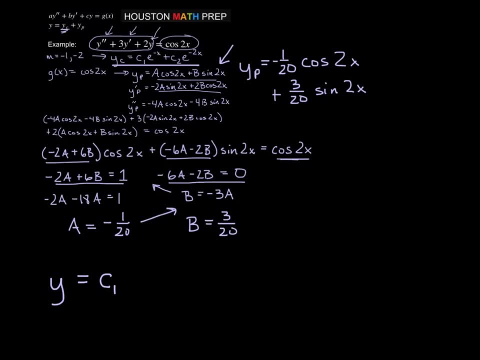 with our y sub c that we got at the very beginning, then we're good to go. So our solution for this one is our complementary function: c1 e to the minus x plus c2 e to the minus 2x. 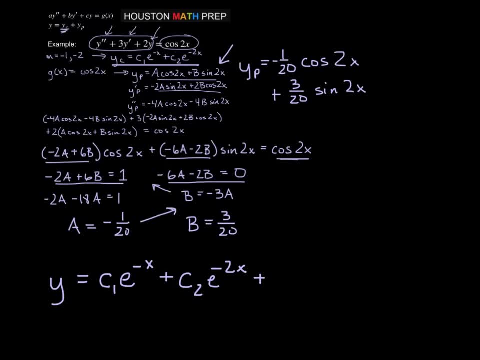 plus our particular solution. I'll go ahead and write here, I guess 3 over 20 sine 2x, since I already wrote the plus sign down, minus 1 over 20, c cosine 2x, So it doesn't matter which order. 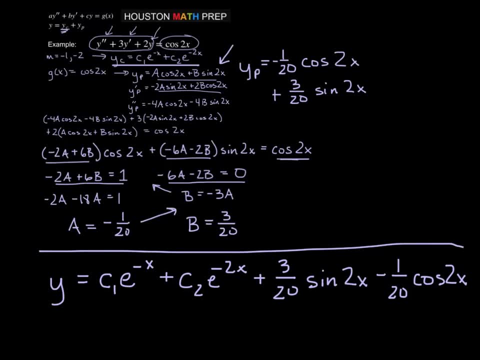 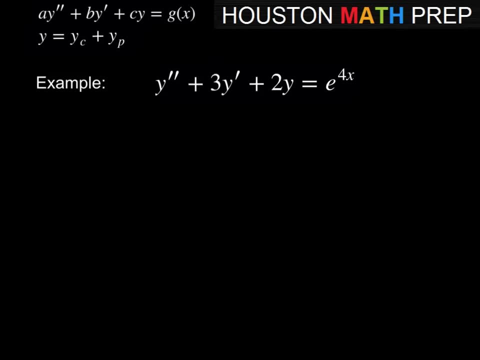 we put those terms in. Alright. and a final example. let's do an exponential one. So again here, exact same left side of the equation. so we're definitely going to get the complementary function c1, e to the minus x. 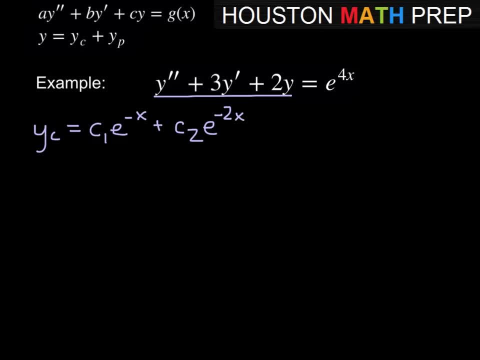 plus c2, e to the minus 2x which we've gotten because we've kept that side the same the whole time. Notice our g of x is e to the 4x. so that tells us that y sub p must be of the form some multiple. 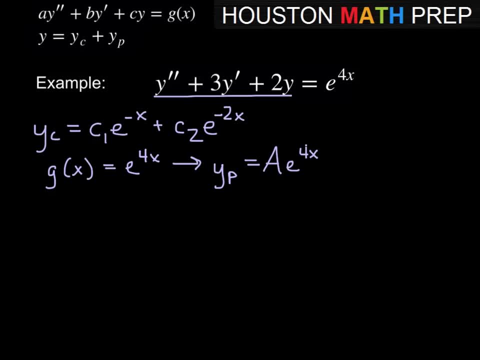 of e to the 4x. Alright derivatives, not too bad. here y prime would be 4a, e to the 4x. y double prime then would be 16, a e to the 4x, If we plug that information in up here. 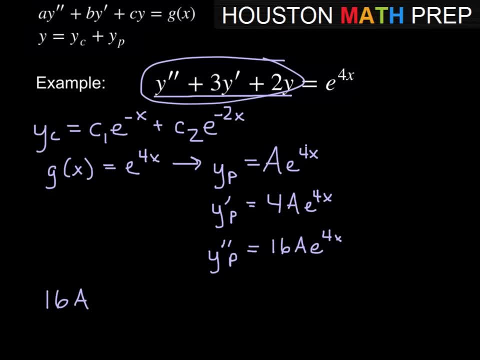 we get the expression 16a e to the 4x plus 3 times y prime, which is 4a e to the 4x plus 2 times y, y is a e to the 4x. 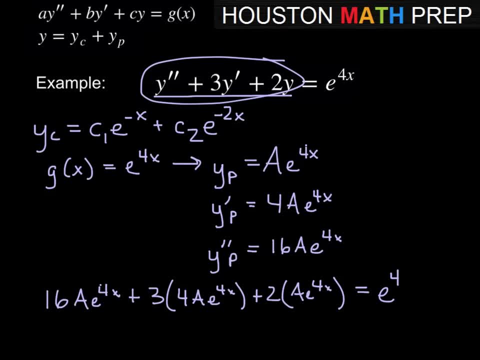 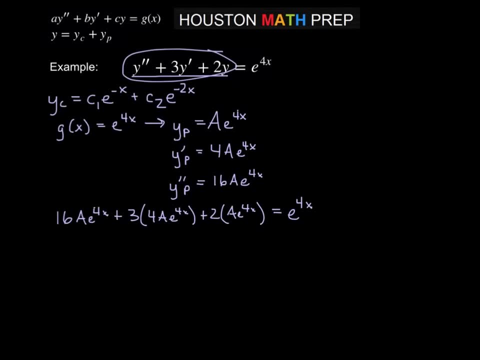 and that's supposed to equal e to the 4x. Alright, so we're almost finished with this one. So, combining all these like terms, so we have 16 here. 3 times 4, that'd be 12 more.